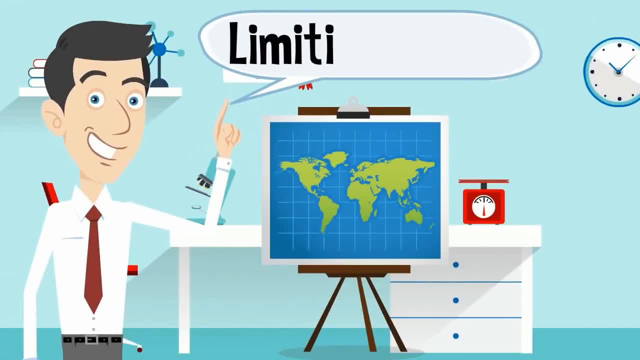 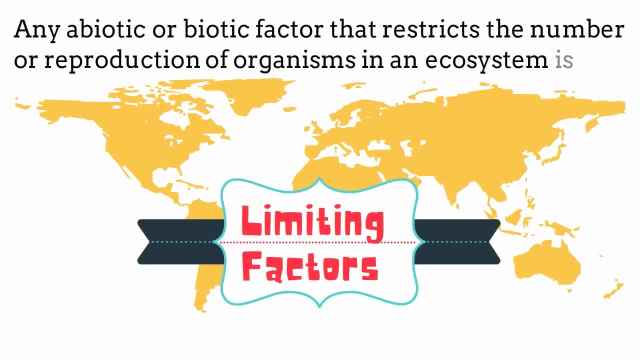 Welcome to MooMooMath and Science. In this video I would like to talk about limiting factors. Any abiotic factor or biotic factor that restricts the number or reproduction of organisms in an ecosystem is called a limiting factor. Take this ecosystem found in the fish. 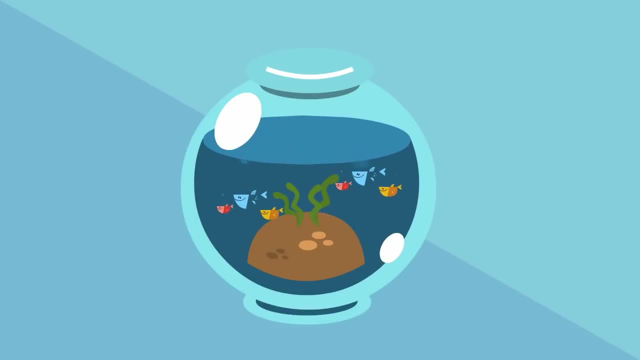 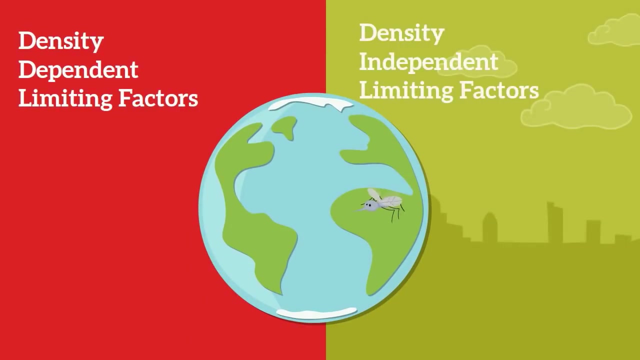 bowl. The limiting factors could be the size of the bowl, the amount of water or the temperature, and any of these can limit the number of fish that can survive in the fish bowl. Limiting factors can be dependent limiting factors and independent limiting factors. Dependent. 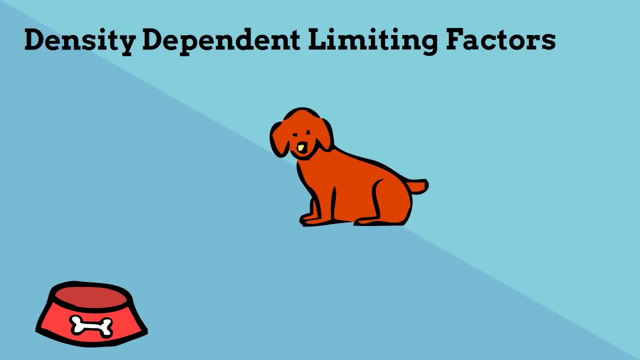 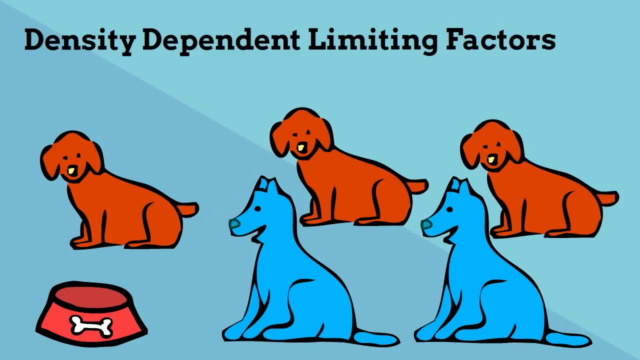 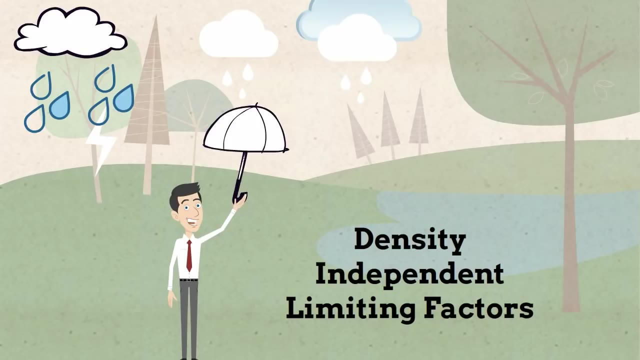 limiting factors depend on the number of organisms. For example, the amount of food available for each organism depends on the number of organisms in this ecosystem. An independent limiting factors does not depend on the number of organisms. For example, the amount of rainfall does not depend on the number of organisms. You 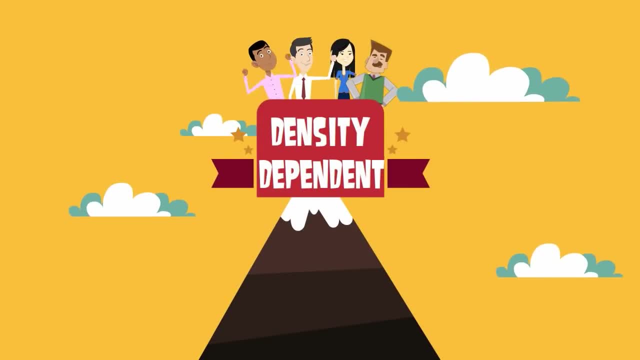 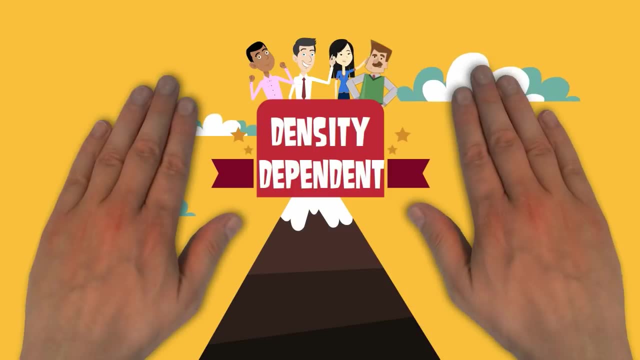 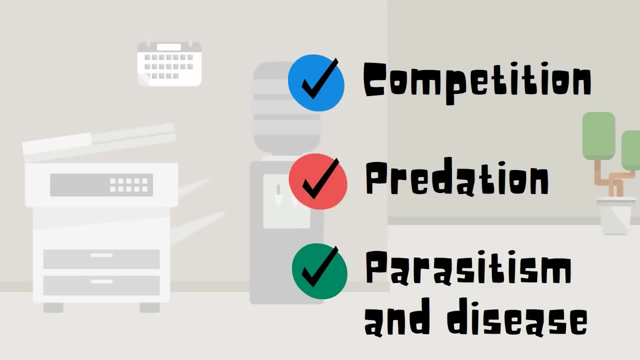 also have density dependent limiting factors, and it is a limiting factor that depends on population size. For example, these could include competition predation, parasitism and disease. Let's look at a list of abiotic limiting factors. This could include sunlight. 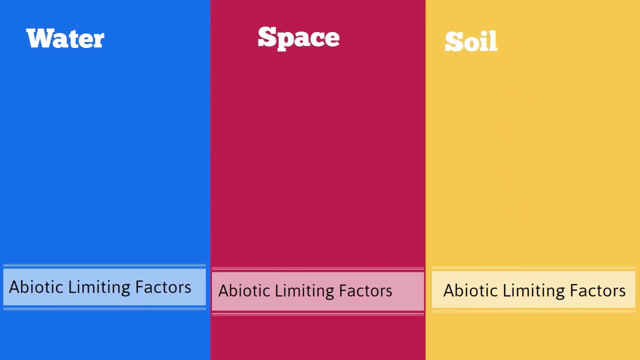 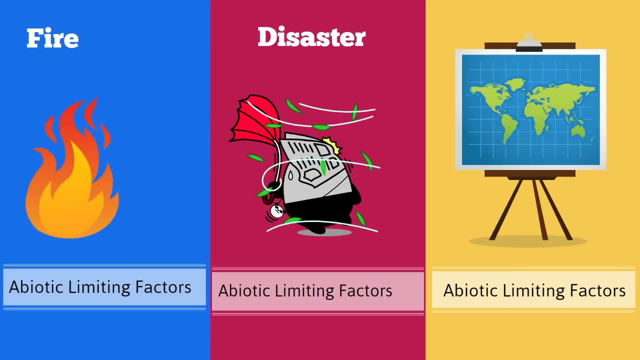 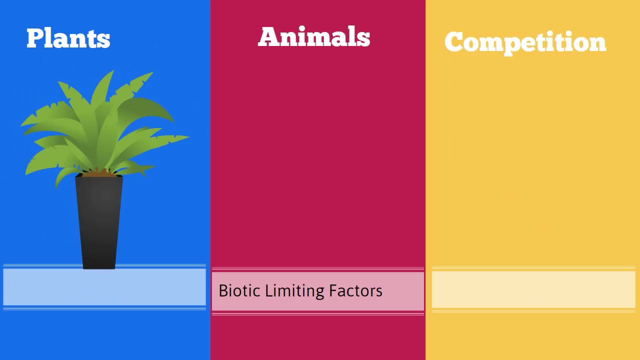 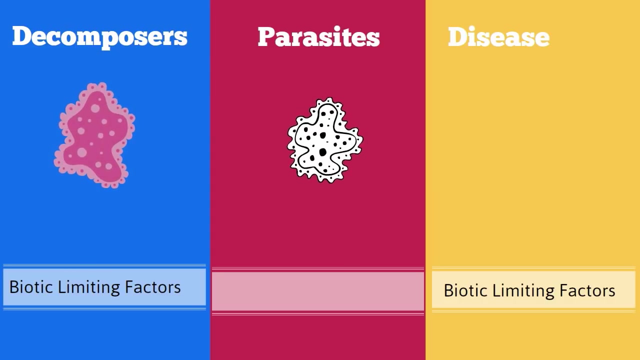 climate, temperature, water, space, soil, chemistry, fire and natural disasters. A list of biotic limiting factors include the number of plants, number of animals, amount of competition, number of decomposers, number of parasites and disease-causing agents. 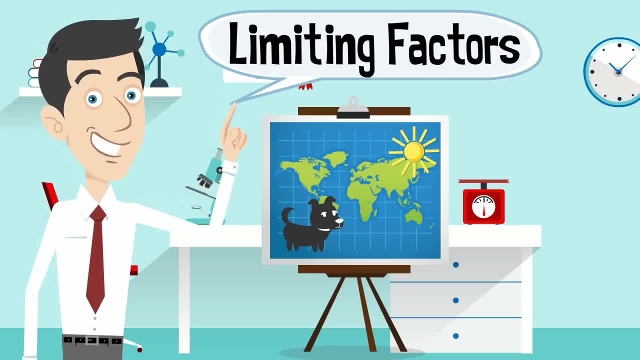 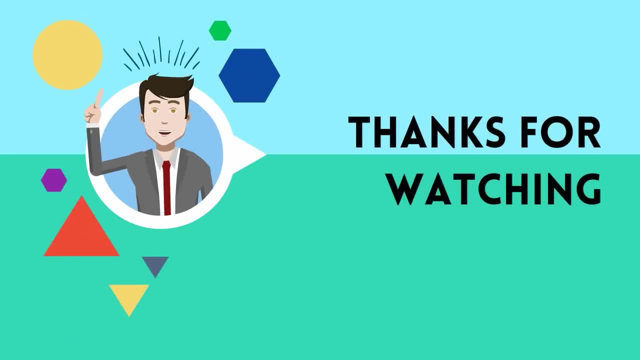 These are biotic and abiotic factors that limit the size, number and reproduction of organisms in an ecosystem.